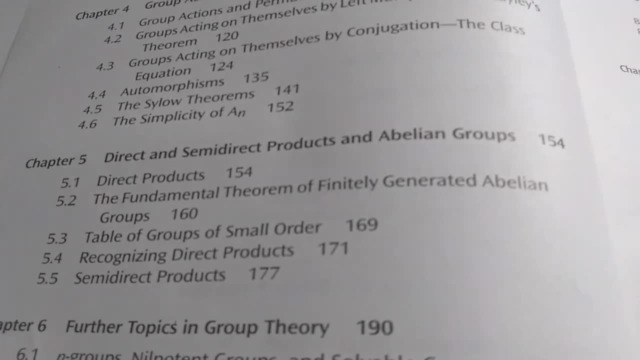 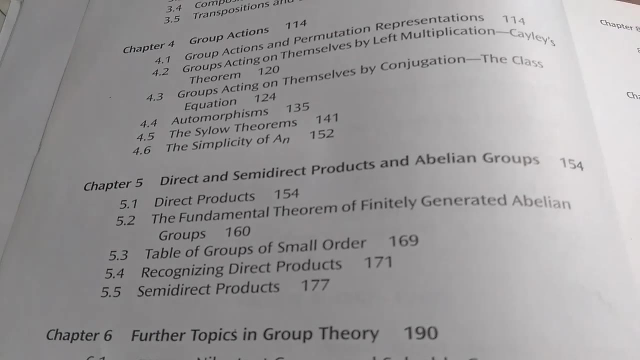 So, and for this. Direct and semi-direct products. I also use this book to help myself learn semi-direct products. Not direct, just semi-direct. 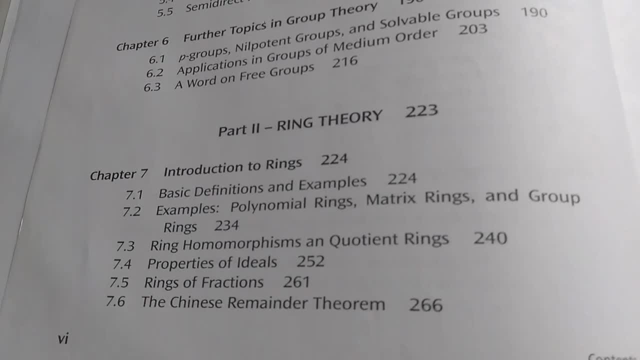 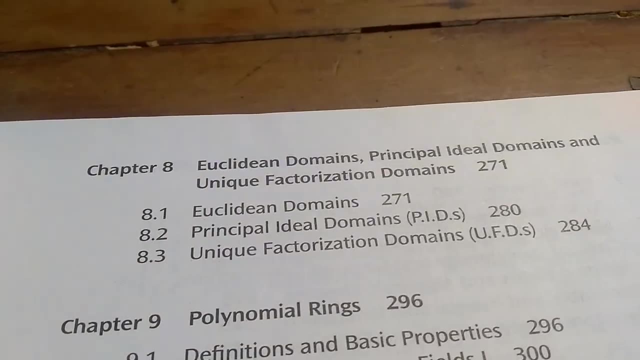 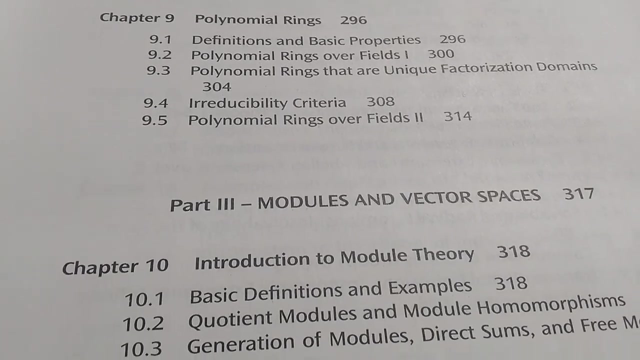 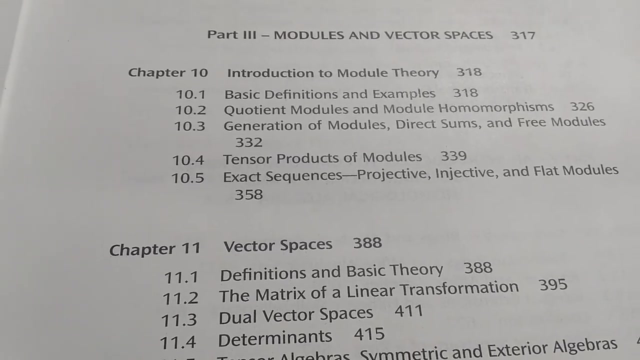 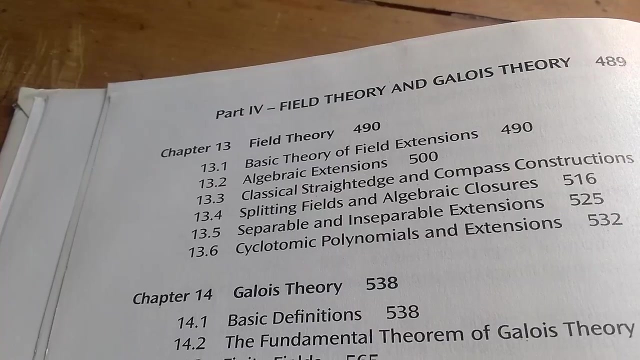 And some more topics. Then he goes into rings. I've actually read the ring theory stuff, including the Chinese remainder theorem. Then he talks about Euclidean domains, PIDs and UFDs, polynomial rings, modules and vector spaces, tensor products of modules, I've also read that section, exact sequences, vector spaces, modules over PIDs, field theory, Galois theory, lots of stuff here. Really good book. 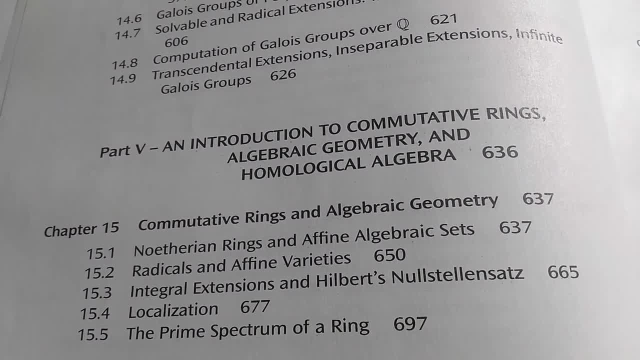 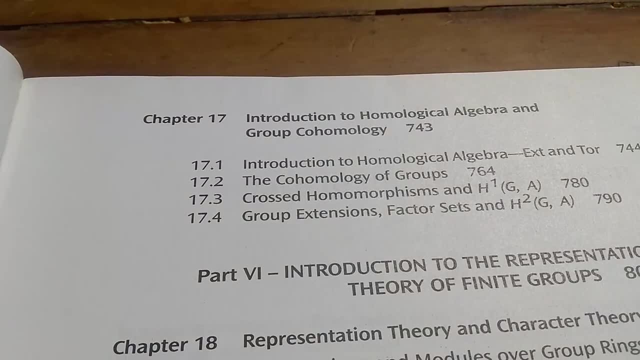 And then he talks about some other stuff, right? Neutharian rings, Artinian rings, really great stuff, homological algebra, and then representation theory and character theory. 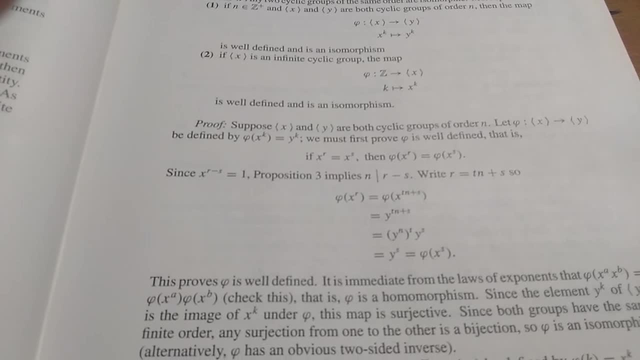 So the textbook is very well written. Dummett and Foote is an excellent book. I have spent a long time reading this book. 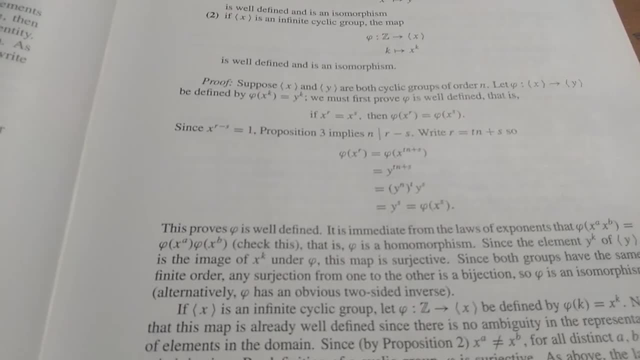 Unfortunately, I was never able to use this book in a course. I think it would have been. 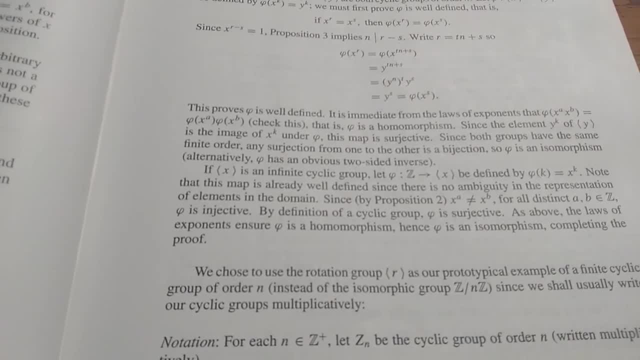 It's a really great book. It's got a lot of information. It reads well. 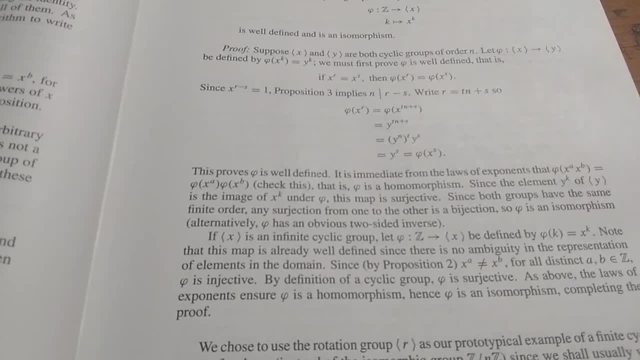 And if you're learning algebra on your own, it's a good book to learn from. It helps to have other books with you. But this one is definitely worth having. 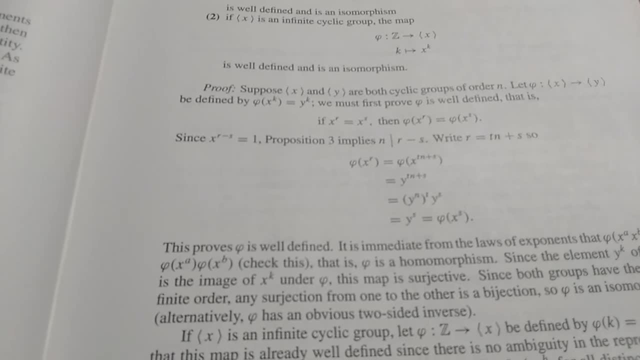 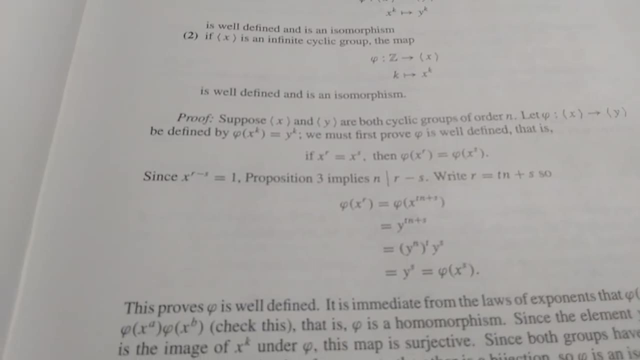 It's worth having this book because it's written at a higher level and it has more information than your typical algebra book. There's so much stuff in here that you can't find in like an undergraduate abstract algebra book. 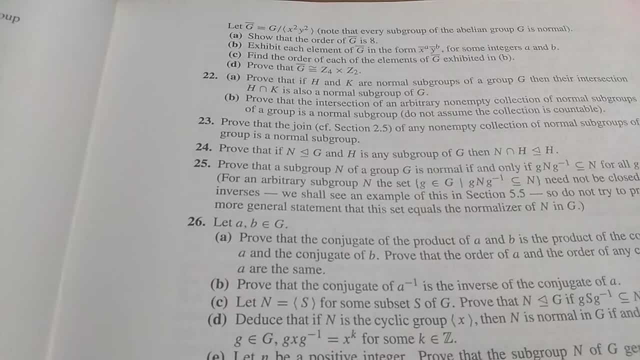 Dummett and Foote has tons of problems. Tons. Each section has a lot of problems. I mean, this is 3.1. We're already up to 34. I think that's it. Let me turn the page. Nope, 43. So, I mean, ridiculous. 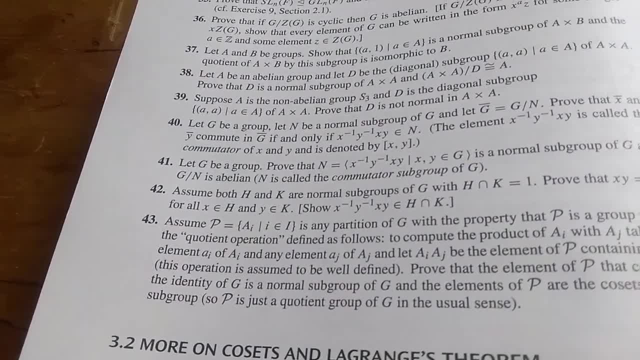 There are so many exercises. So if you're looking for practice, there is no shortage of that in this book. Again, the readability of this book is quite good. 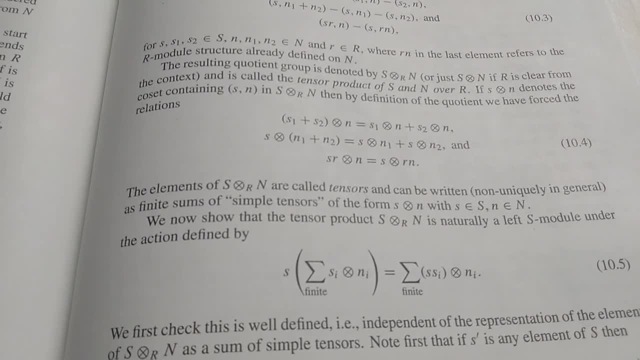 It's a good book and it has a lot of topics that you can't find. And other textbooks. 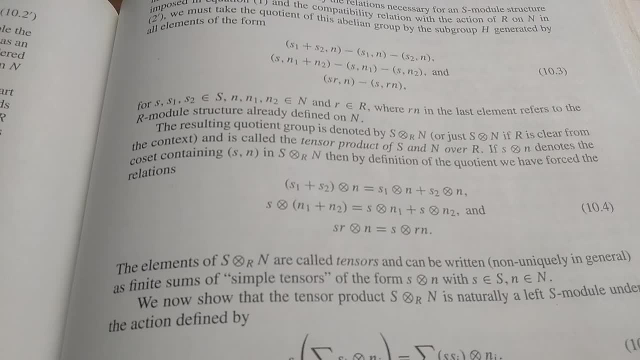 So that alone makes it worth having. My only regret with this book is that I didn't buy a new copy.